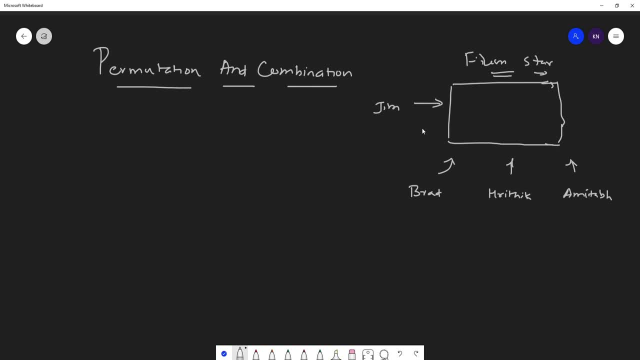 you know. so, Jim Carrey, and let's consider that you also have Dwayne Johnson. I'll just say it as Rock. I hope everybody knows it. so suppose I have 1,, 2,, 3,, 4,, 5, 5 people again. let's add one more. 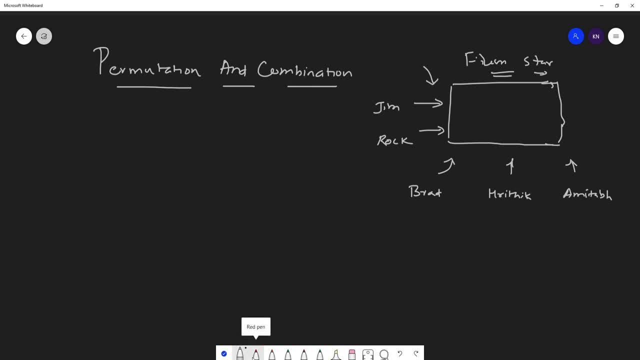 hero, probably anything we can actually take. let's take our Indian movies hero. we have Shah Rukh Khan. okay, Shah Rukh Khan, okay. so these are some of the popular actors. okay, now I will give a task to a person, like I'll give him a book and say him that once you enter the house, 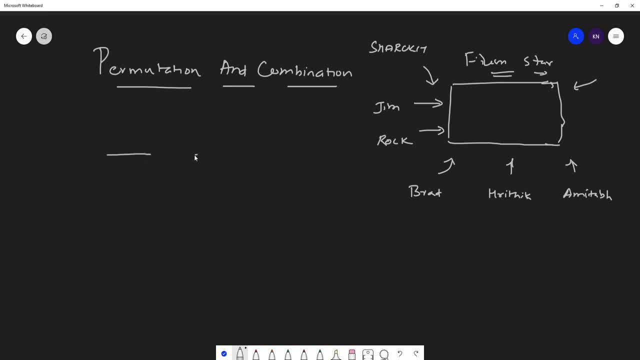 whichever is the first three actors, please note down their name. okay, like this. note down their name, or probably you just have to make a record of it. okay, now, when this particular task is actually given. suppose the person enters into the house. okay, over here, you know that there. 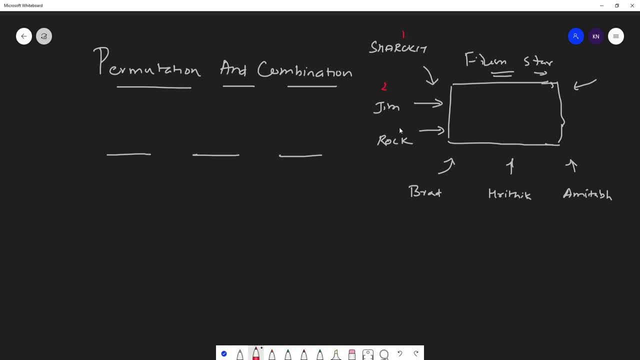 are six actors if I talk about this. this is 1,, 2,, 3,, 4,, 5,, 6, obviously the first option when he's actually seeing any of the actor. right, obviously there will be around six options, initially, right in the second record when he's actually noting down. 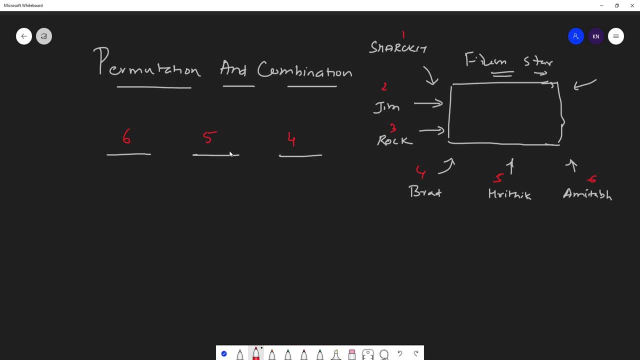 the second record, then probably there will be five options and last there will be around four options. right now this are the possible set of options that we may probably have when they actually want to see, suppose, if he's trying to record the actor that he sees right now. these 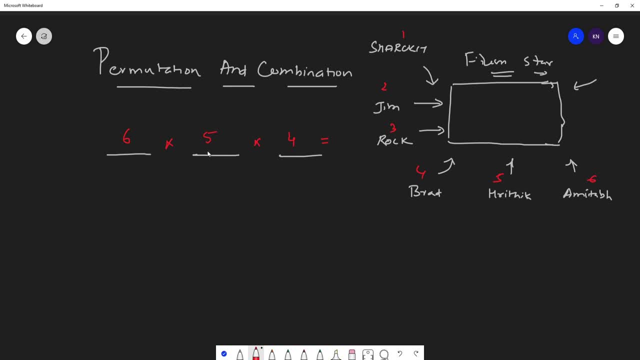 are all the possible options that he may have. now, when I say about possible options, I'm also talking about the order. I'll talk about this here. this, I'll say: this order matters over here. okay, now let's compute the total of this like: what are the possible options? 6 multiplied by 5. 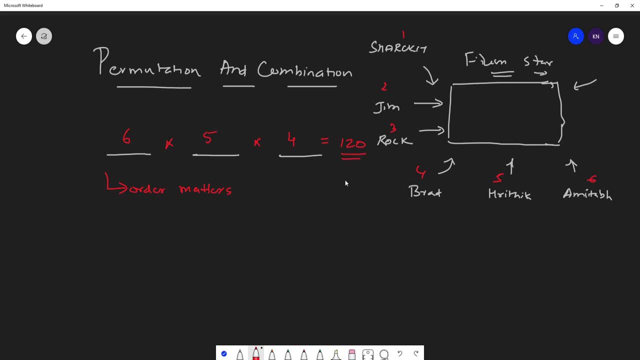 multiplied by 4, it is nothing but 120 options. okay, now this basically means that suppose let's consider that probably I want to record this in the initial time when I'm not selecting anyone- I may have six possible options, then five possible options, then four possible options. 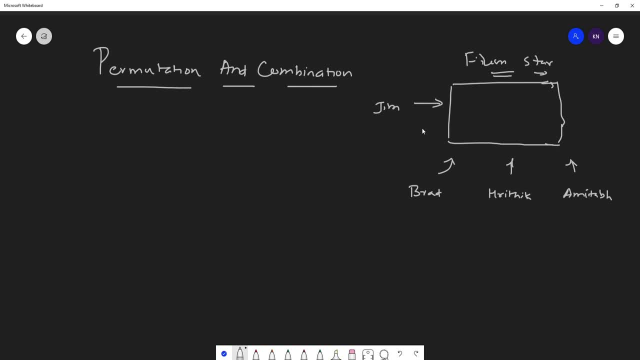 you know. so, Jim Carrey, and let's consider that you also have Dwayne Johnson. I'll just say it as Rock. I hope everybody knows it. so suppose I have 1,, 2,, 3,, 4,, 5, 5 people again. let's add one more. 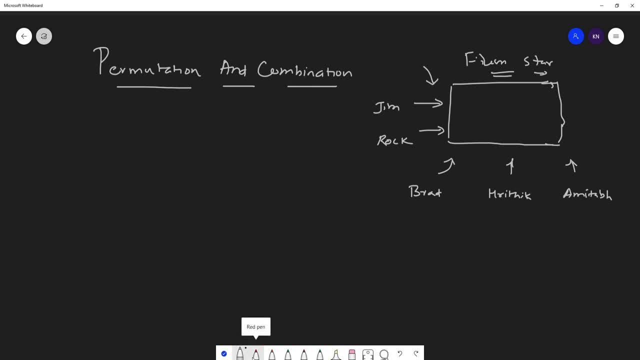 hero, probably anything we can actually take. let's take our Indian movies hero. we have Shah Rukh Khan. okay, Shah Rukh Khan, okay. so these are some of the popular actors. okay, now I will give a task to a person, like I'll give him a book and say him that once you enter the house, 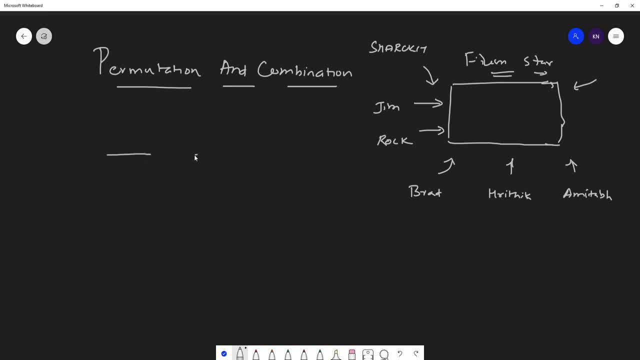 whichever is the first three actors, please note down their name. okay, like this. note down their name, or probably you just have to make a record of it. okay, now, when this particular task is actually given. suppose the person enters into the house. okay, over here, you know that there. 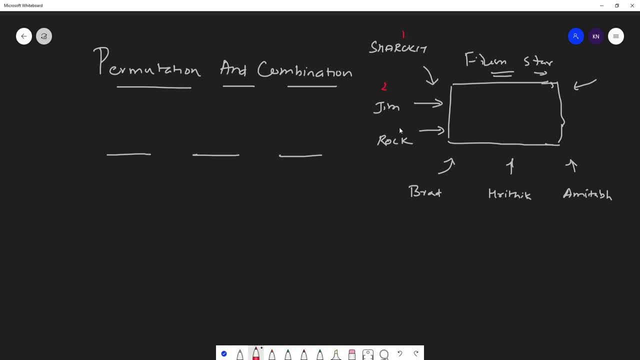 are six actors if I talk about this. this is 1,, 2,, 3,, 4,, 5,, 6, obviously the first option when he's actually seeing any of the actor. right, obviously there will be around six options, initially, right in the second record when he's actually noting down. 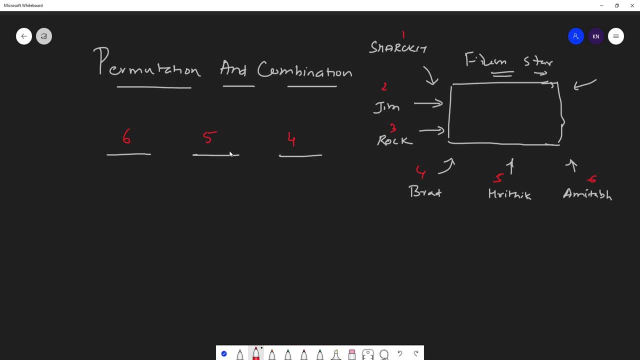 the second record, then probably there will be five options and last there will be around four options. right now this are the possible set of options that we may probably have when they actually want to see, suppose, if he's trying to record the actor that he sees right now. these 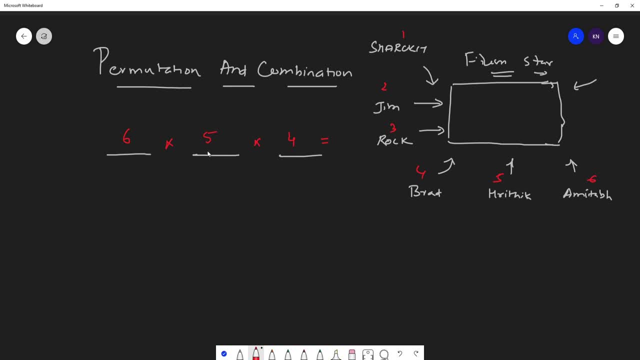 are all the possible options that he may have. now, when I say about possible options, I'm also talking about the order. I'll talk about this here. this, I'll say: this order matters over here. okay, now let's compute the total of this like: what are the possible options? 6 multiplied by 5. 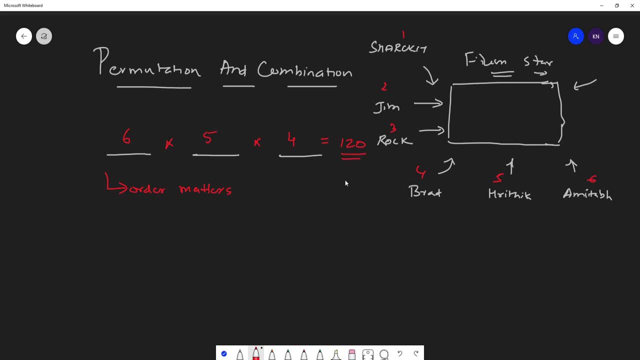 multiplied by 4, it is nothing but 120 options. okay, now this basically means that suppose let's consider that probably I want to record this in the initial time when I'm not selecting anyone- I may have six possible options, then five possible options, then four possible options. 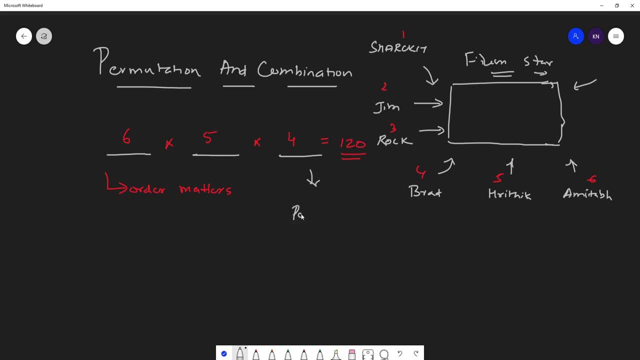 this entirely is called as permutation, you know. so I'm basically noting down all the possibilities, all the possibilities of selecting or seeing a specific actor from this particular house, and over here the order matters why. I'll tell you guys, suppose, if I see the first hero as Rock, and then probably I'll see Shah Rukh, or let me. 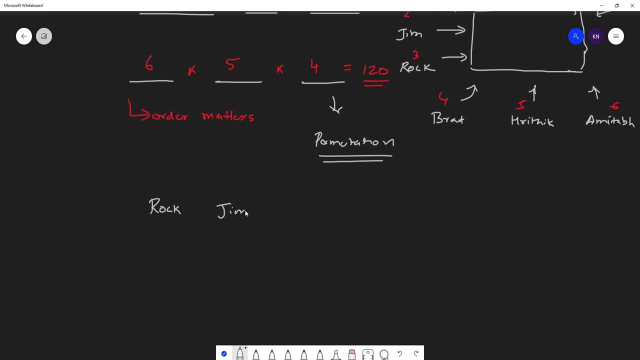 just write some Hollywood heroes. okay, probably I'll write Jim Carrey and then I'll write Brad Pitt, okay, so this may be one combination. the next combination can also be Jim Rock, Brad, right, so I may have multiple combination like this and remember over here: 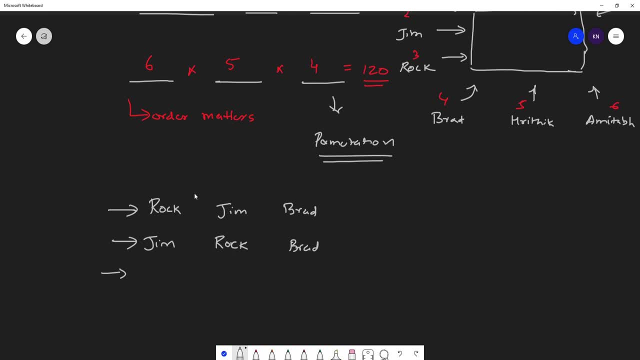 the order will not matter. now, when I say order will not matter, that basically means I have taken the same people right- Rock, Jim, Brad- but here I've just changed the order right, but I have to count this as separate permutations, right? so like this we will be using all the possible. 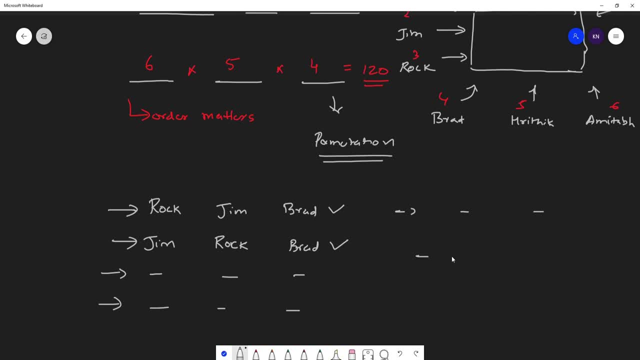 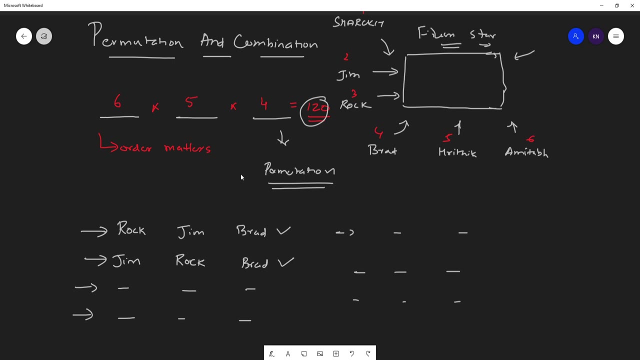 combination, and probably after having all the possible combination, we may have this many number of actors, and this entirely is called as permutations. okay, permutations now, very, very simple guys. these are the possible options, because I'll make you understand what is the exact difference between. 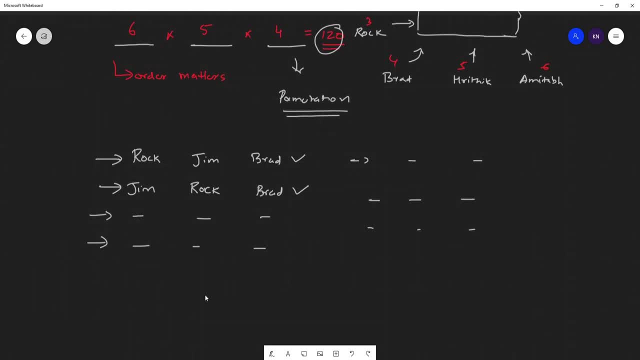 permutation and combination too. okay, now, if I really want to define this permutation formula, I can basically write it as: so: permutation is usually given as npr. and this is basically given as n factorial divided by n minus r factorial. now, what is this? n, n is nothing but the total. 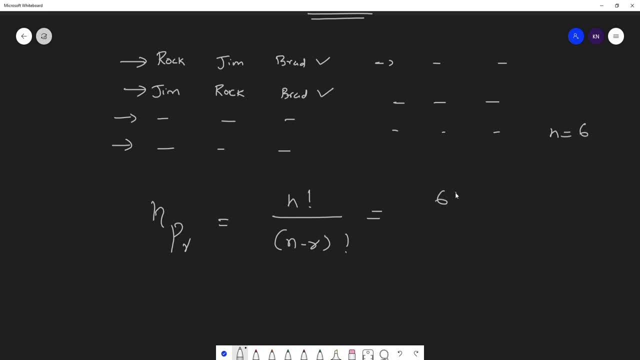 number of actors that were present. so over there it was 6, so I will write 6 factorial divided by n minus r. what is r over here? r basically means how many number of records. I had right, probably 3, and I have to take all the possible combination. so here I will basically write. 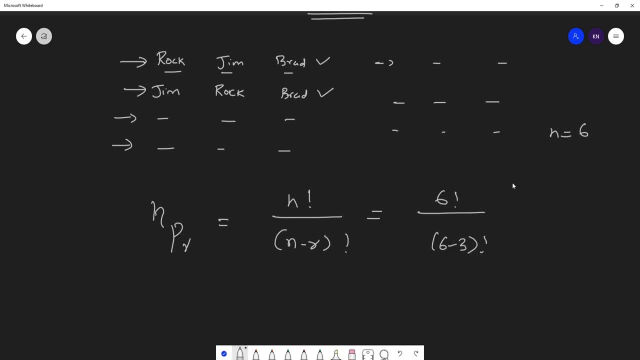 very, very simple: 6 minus 3 factorial. right now I can basically write 6 multiplied by 4 multiplied by 3 factorial, and this will be actually 3 factorial. when I cancel this right, 3 factorial, 3 factorial is gone. the total number. 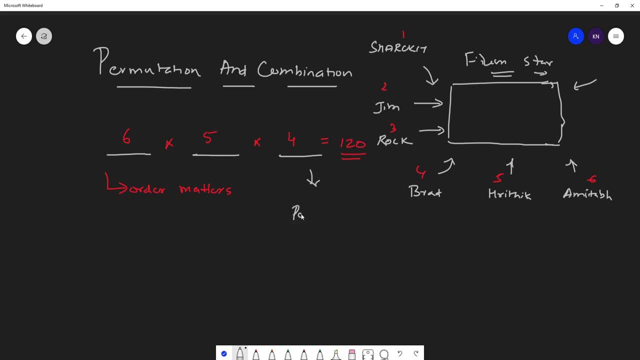 this entirely is called as permutation, you know. so I'm basically noting down all the possibilities, all the possibilities of selecting or seeing a specific actor from this particular house, and over here the order matters why. I'll tell you guys, suppose, if I see the first hero as Rock, and then probably I'll see Shah Rukh, or let me. 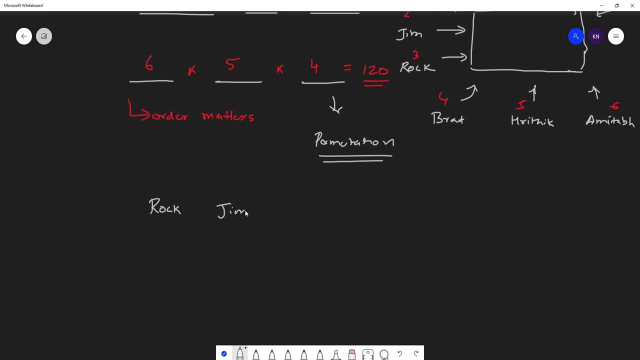 just write some Hollywood heroes. okay, probably I'll write Jim Carrey and then I'll write Brad Pitt, okay, so this may be one combination. the next combination can also be Jim Rock, Brad, right, so I may have multiple combination like this and remember over here: 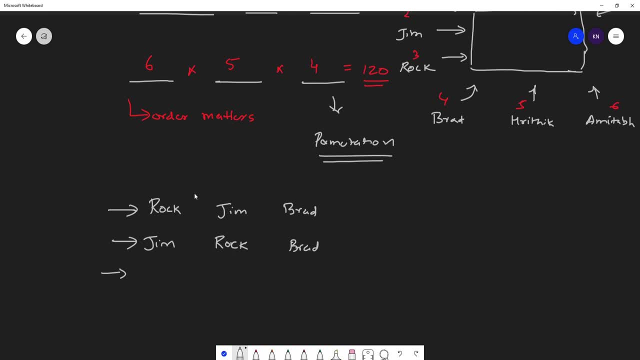 the order will not matter. now, when I say order will not matter, that basically means I have taken the same people right- Rock, Jim, Brad- but here I've just changed the order right, but I have to count this as separate permutations, right? so like this we will be using all the possible. 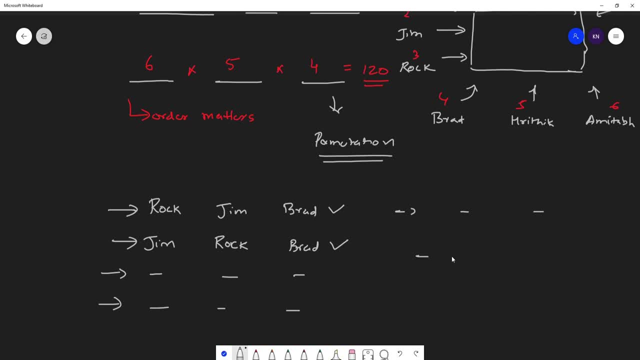 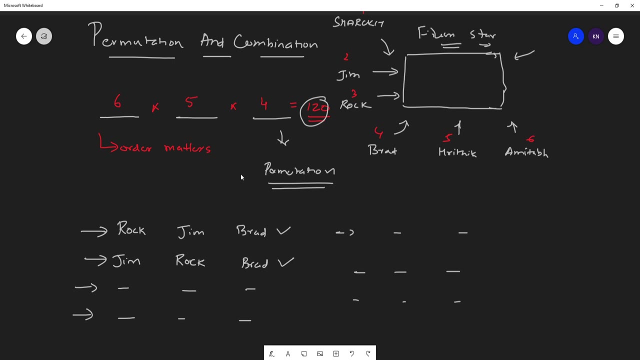 combination, and probably after having all the possible combination, we may have this many number of actors, and this entirely is called as permutations. okay, permutations now, very, very simple guys. these are the possible options, because I'll make you understand what is the exact difference between. 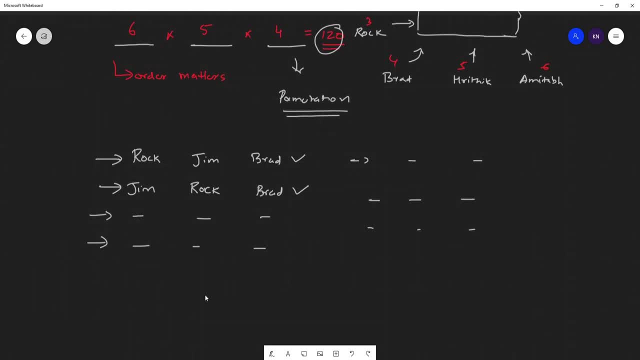 permutation and combination too. okay, now, if I really want to define this permutation formula, I can basically write it as: so: permutation is usually given as npr. and this is basically given as n factorial divided by n minus r factorial. now, what is this? n, n is nothing but the total. 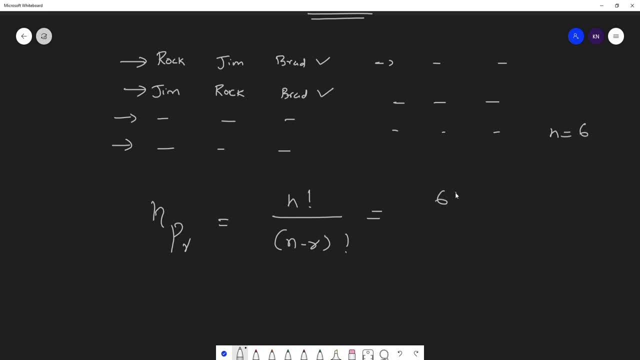 number of actors that were present. so over there it was 6, so I will write 6 factorial divided by n minus r. what is r over here? r basically means how many number of records. I had right, probably 3, and I have to take all the possible combination. so here I will basically write. 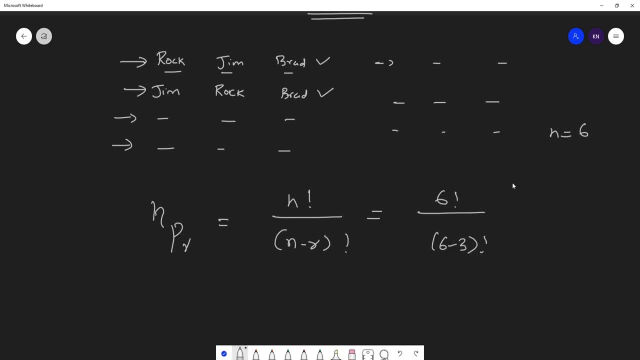 very, very simple: 6 minus 3 factorial. right now I can basically write 6 multiplied by 4 multiplied by 3 factorial, and this will be actually 3 factorial. when I cancel this right, 3 factorial, 3 factorial is gone. the total number. 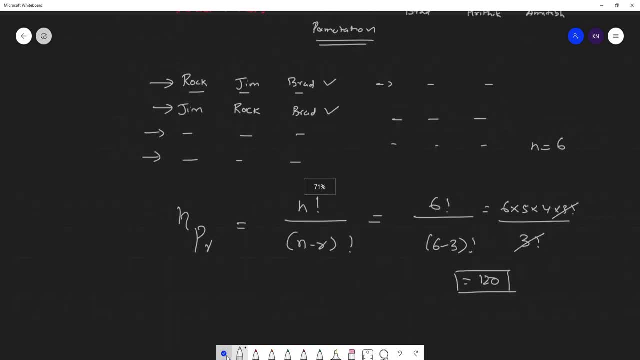 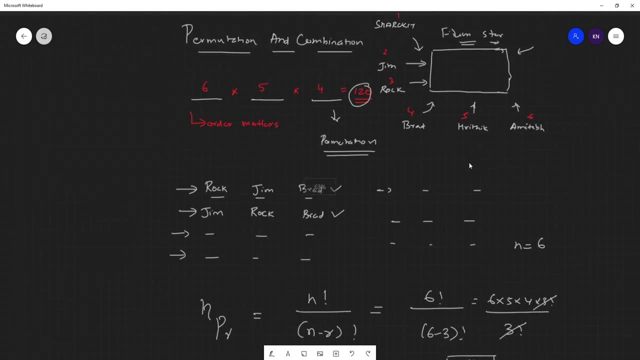 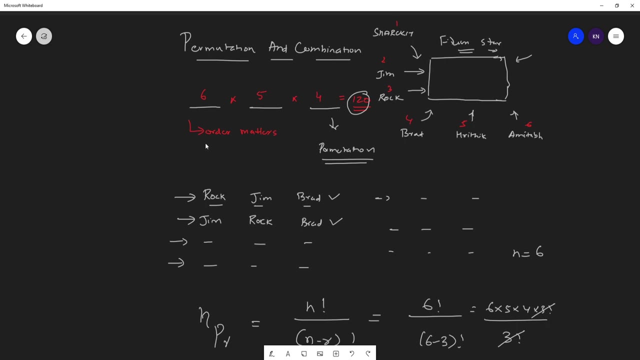 that I'm going to get 120, and that is the same output. we got over here right with respect to all the possible combination. so I hope you have got an idea about permutation. it's like selecting all the possible options and over there the order is every order. every order is basically: 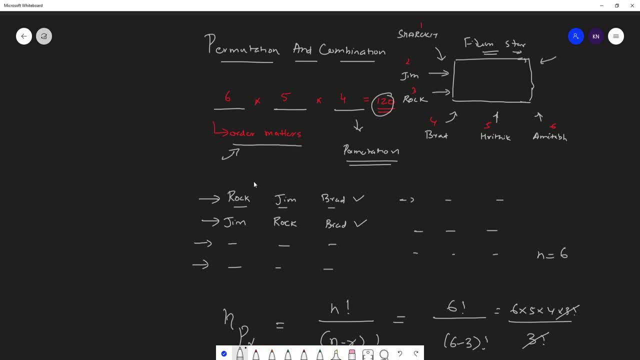 treated as a separate count. now, when I say about order, suppose I take Rock, Jim and Brad. the same people can be, you know, shifted here and there, and probably that can also be taken as another option. okay, now, this was with respect to permutation. I hope everybody. 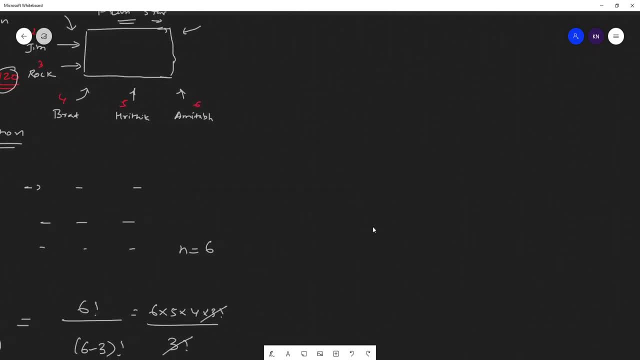 has got this specific idea. now let's understand about combination and we'll also understand about the formula. now, in combination, as the number, as the sorry, as the name says: combination. okay, here the order does not matter. okay, now, when I say add, order does not matter. see, 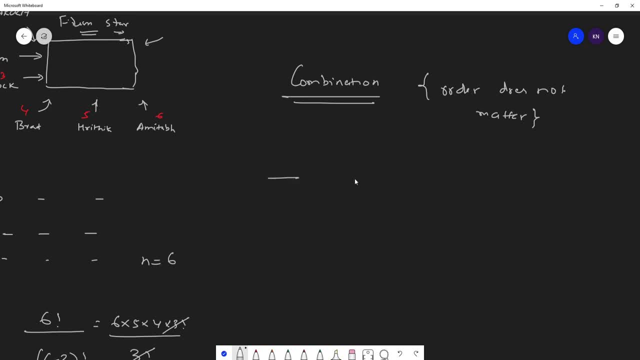 when I say about combination in this three cases, suppose I am selecting Rock, probably I'm selecting Jim and probably I'm selecting Brad Pitt. okay, so this may be one combination. okay, one combination there. now, if I take the same people and just shift them. 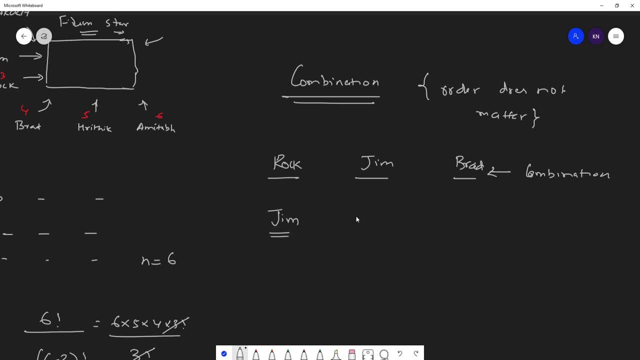 in different orders. now probably, if I take them Jim or Rock or Brad, in this particular scenario this will be a different permutation, but this cannot be a different combination because, understand, we are taking the same number of people, you know same. 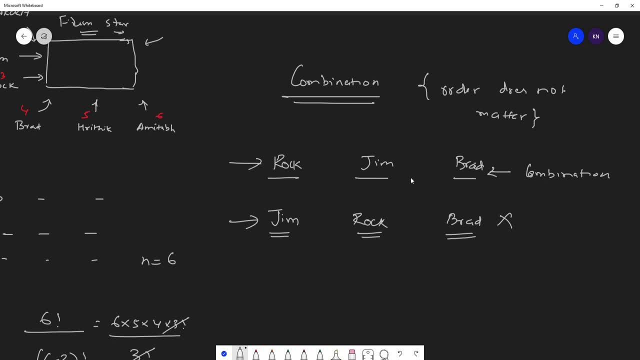 same people which where I have actually combined them together. you know, this is a unique combination and over here, even though I don't, I change this specific order. okay, it won't matter. we cannot take this as our second combination. this will be one combination only, right, so with? 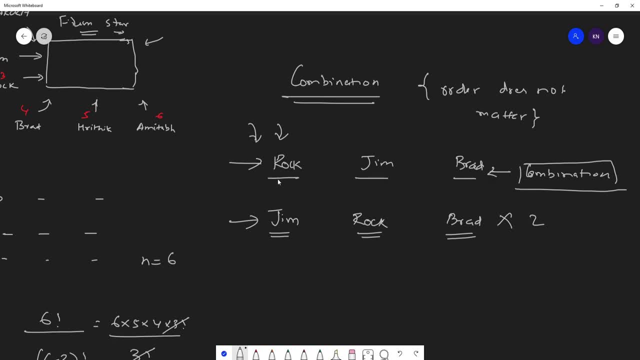 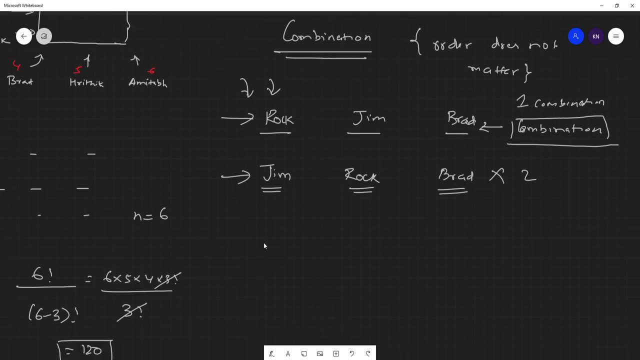 respect to this, all people you know. however you move the position or shuffle the position, this will be treated as one combination, right? this is a very important thing to understand now. based on this, the formula of combination basically changes. 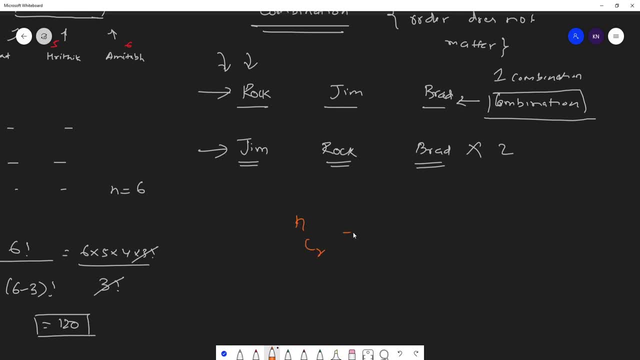 like this: okay, I can basically write the combination formula as: ncr divided by n factorial r factorial and n minus r factorial. here, obviously, n- we know it's 6- factorial r factorial is nothing but 3, because we have 3 different position, and then n minus 3 is nothing. 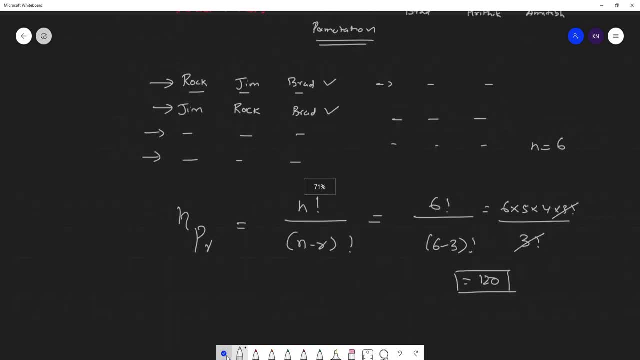 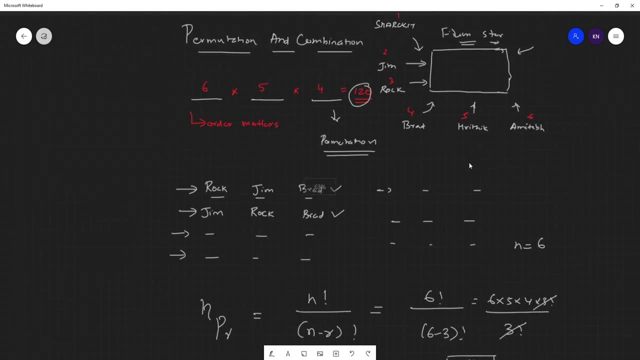 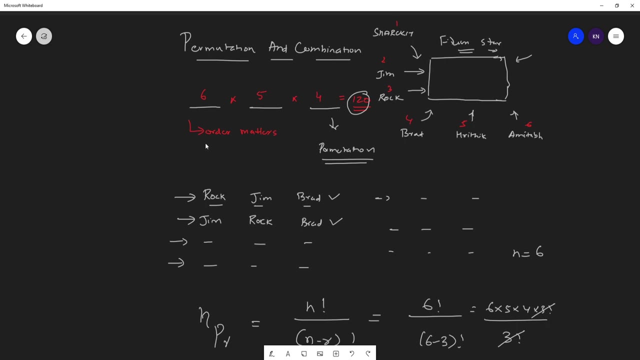 that I'm going to get 120, and that is the same output. we got over here right with respect to all the possible combination. so I hope you have got an idea about permutation. it's like selecting all the possible options and over there the order is every order. every order is basically: 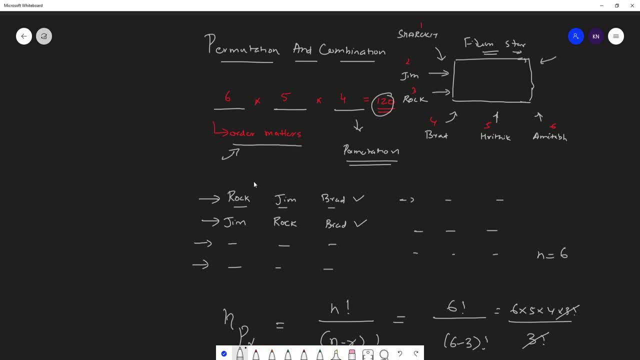 treated as a separate count. now, when I say about order, suppose I take Rock, Jim and Brad. the same people can be, you know, shifted here and there, and probably that can also be taken as another option. okay, now, this was with respect to permutation. I hope everybody. 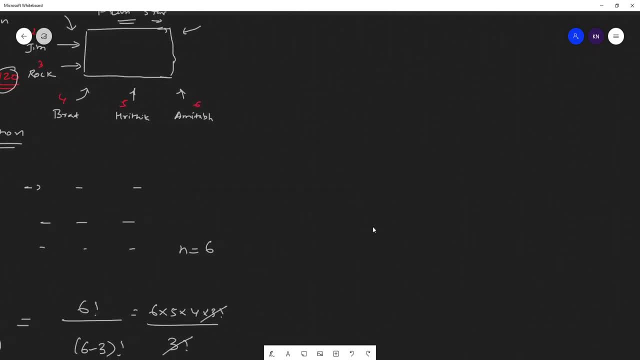 has got this specific idea. now let's understand about combination and we'll also understand about the formula. now, in combination, as the number, as the sorry, as the name says: combination. okay, here the order does not matter. okay, now, when I say add, order does not matter. see, 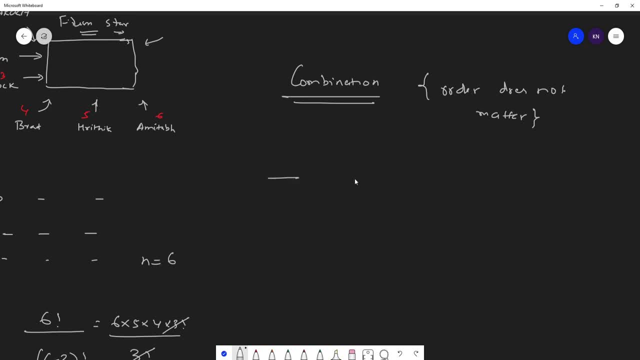 when I say about combination in this three cases, suppose I am selecting Rock, probably I'm selecting Jim and probably I'm selecting Brad Pitt. okay, so this may be one combination. okay, one combination there. now, if I take the same people and just shift them. 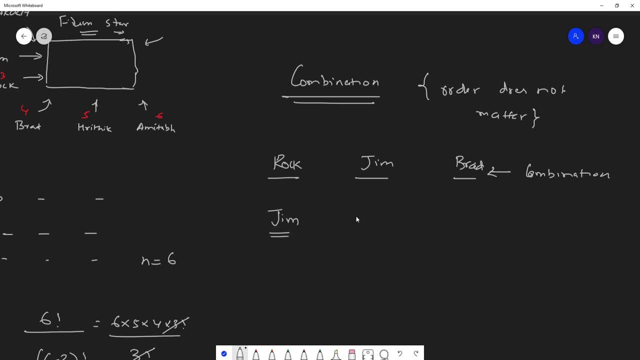 in different orders. now probably, if I take them Jim or Rock or Brad, in this particular scenario this will be a different permutation, but this cannot be a different combination because, understand, we are taking the same number of people, you know same. 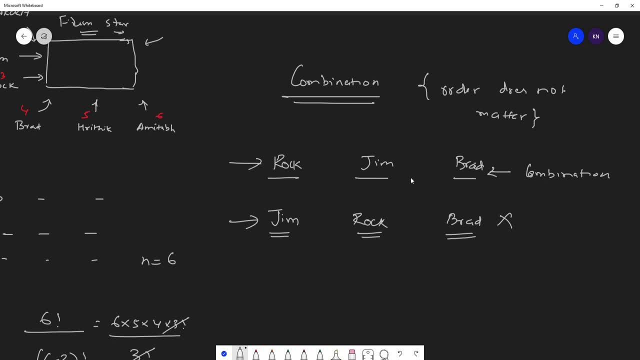 same people which where I have actually combined them together. you know, this is a unique combination and over here, even though I don't, I change this specific order. okay, it won't matter. we cannot take this as our second combination. this will be one combination only, right, so with? 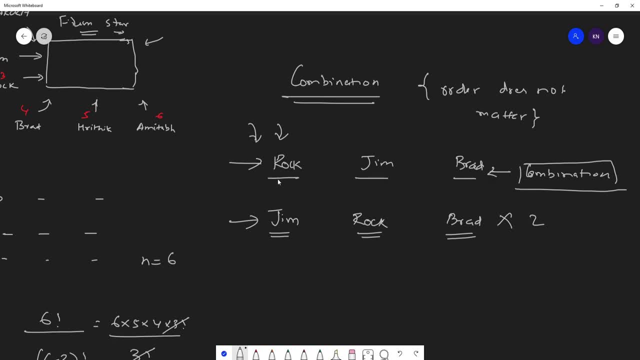 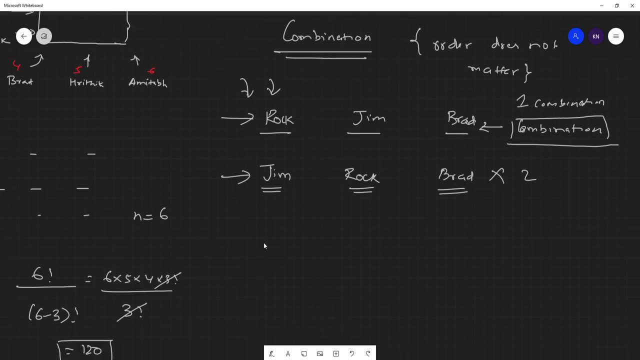 respect to this, all people you know. however you move the position or shuffle the position, this will be treated as one combination, right? this is a very important thing to understand now. based on this, the formula of combination basically changes. 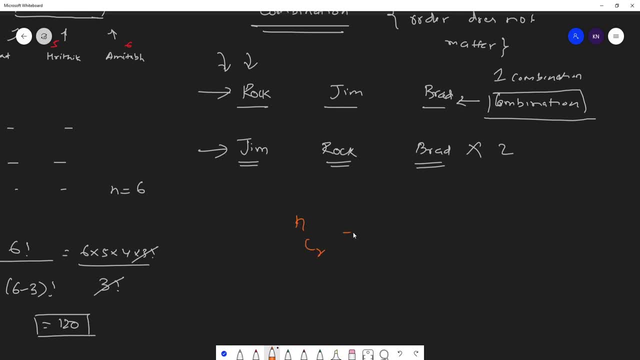 like this: okay, I can basically write the combination formula as: ncr divided by n factorial r factorial and n minus r factorial. here, obviously, n- we know it's 6- factorial r factorial is nothing but 3, because we have 3 different position, and then n minus 3 is nothing. 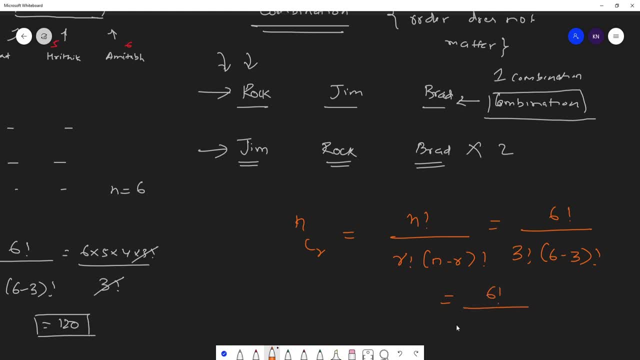 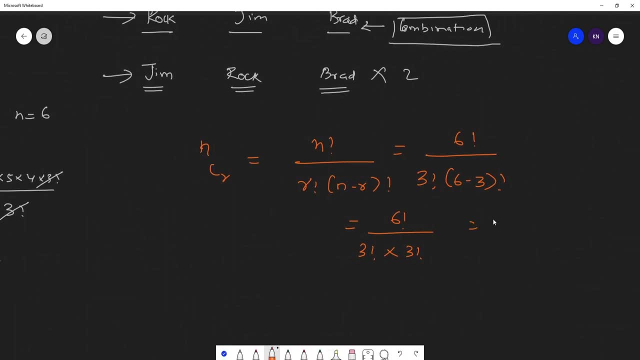 but 6 minus 3 factorial. now, if I try to make this, it is nothing but 3 factorial multiplied by 3 factorial. okay, and if I do this specific calculation, it will be nothing but 6 multiplied by 4, multiplied by 3 factorial, divided by 3 into 2, into 1, multiplied by 3. 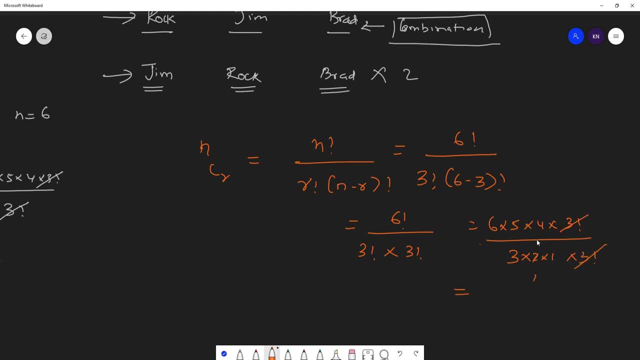 factorial. this 3 factorial and 3 factorial will get cancelled. and here I will be writing: 2, 1's are 3, 3, so the total unique combination will be 20, right, so based on permutation, for the same. 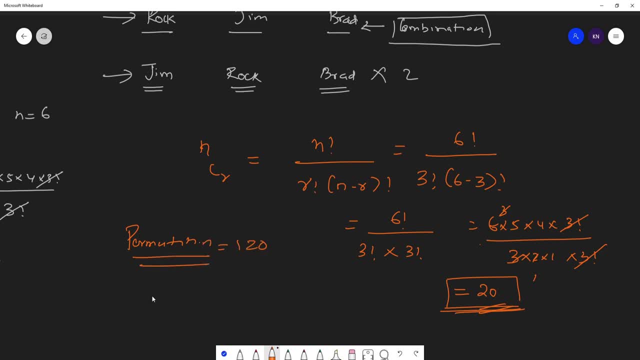 problem statement. we saw where the order mattered. our answer was 120, and obviously combination will be less than permutation, because here it does not matter, because once the order is taken with the name, same element or same people. 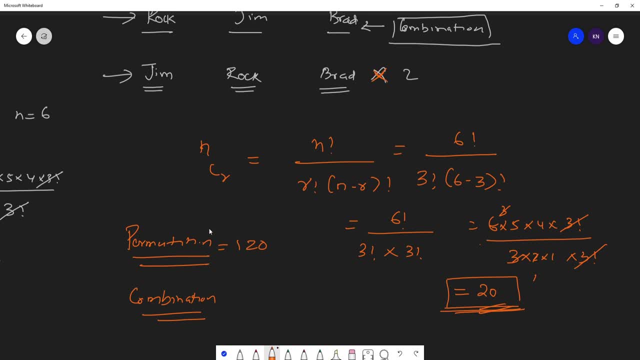 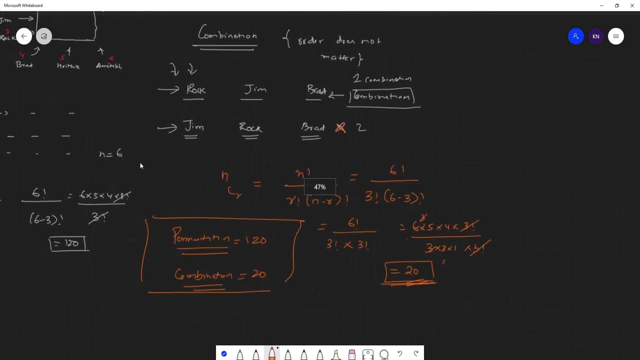 if you try to again shuffle this position, this will not be treated as a second combination. so here I have actually got a 20, so I hope you have understood this video. guys, this is very, very much important to understand the basic difference and based on that, 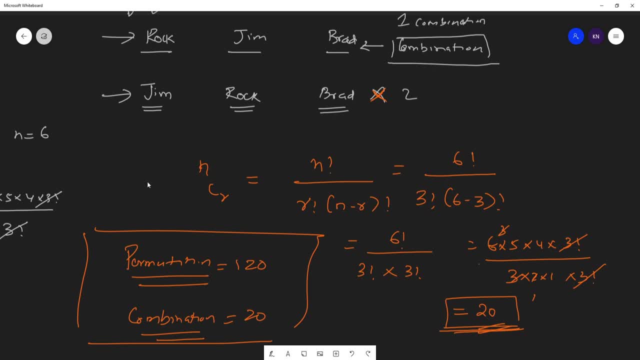 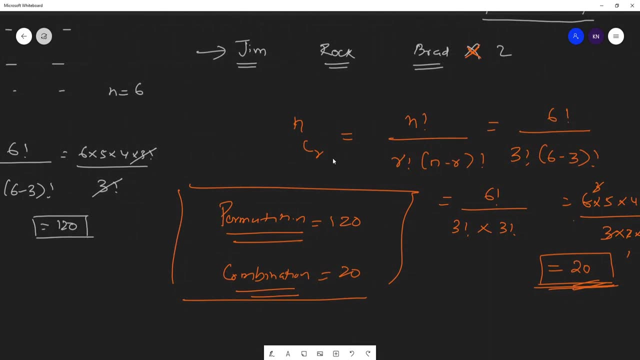 you will be able to understand and remember this particular formula also, right, very, very simple formula: npr. this is for permutation: n factorial divided by n minus r factorial, and this is basically combination ncr, which is equal to n factorial divided by r factorial, multiplied by n minus r factorial. 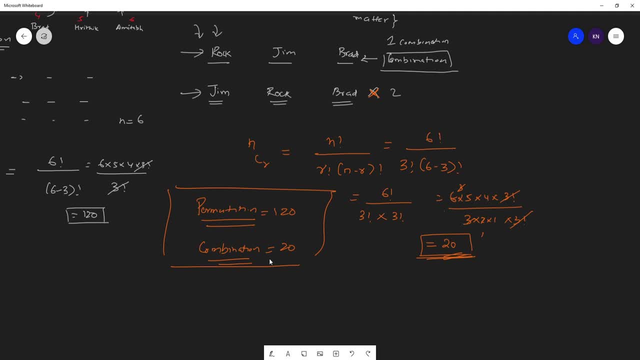 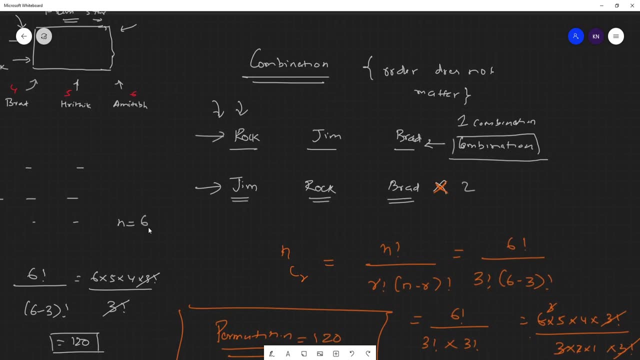 so because of this here you will definitely say that permutation will be sorry, combination will be less than permutation. okay, and obviously in permutation, order matters and in combination, order does not matter. so these are the important things that you really need to remember. 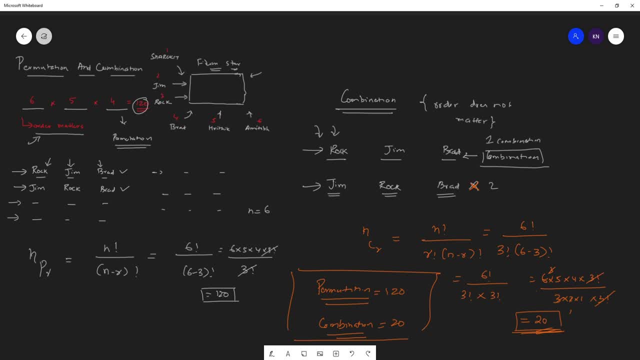 and definitely by just understanding this much, you will be able to solve any kind of problems. okay, so this was the video regarding permutation and combination. I hope you liked it. if you liked it, please do make sure that you subscribe the channel. 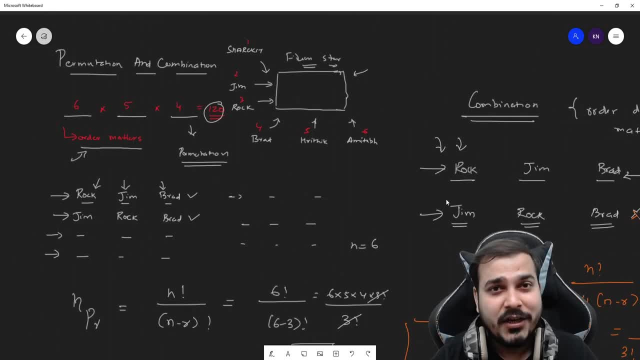 press the bell notification icon. it will motivate me to upload more and more videos. I'll see you all in the next video. have a great day. thank you, one doll, bye-bye.